hopefully you guys are writing small enough. I'm going to try to do it over here just to see if I can do it. Okay, so I'm going to try to do it over here just to see if I can do it. I'm going to try to do it over here just to see if I can do it. 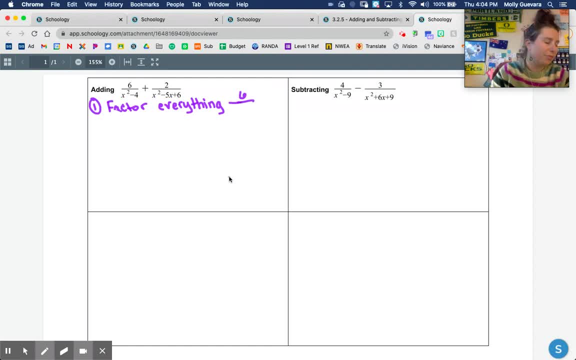 Okay, so I have six on top. Then I have x squared minus four. This is a perfect square, so this factors to x plus two, x minus two. Okay, then I'm adding, Two does not factor, so it's going to stay on the top. 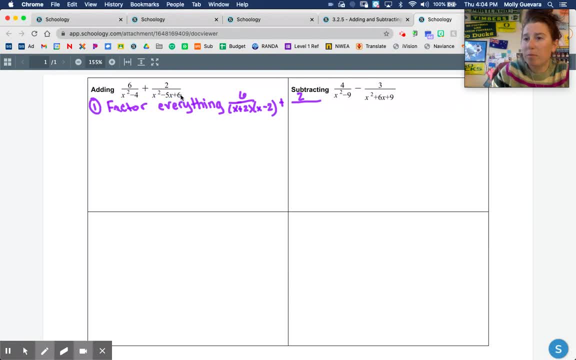 And then x squared minus five, x plus six. So I want two numbers that multiply to positive six and add to negative five, And so that's going to give me x minus three, And so that's going to give me x plus three, x plus two. 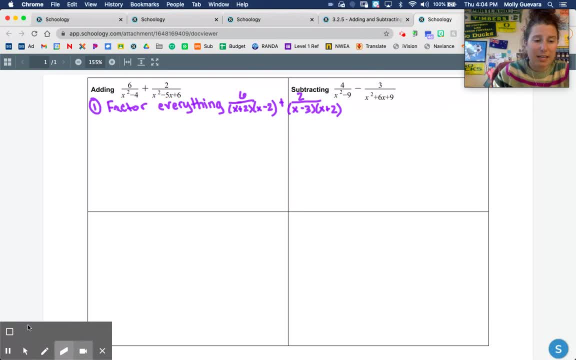 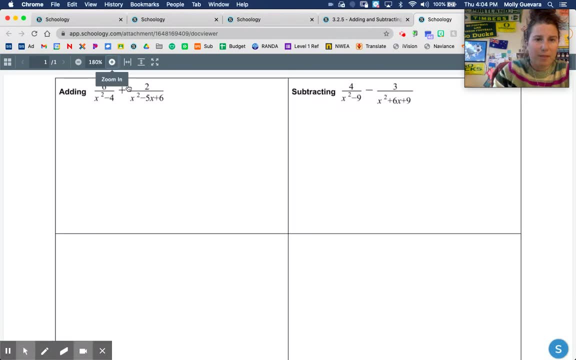 So that's my first step is I want to factor everything. Okay, and I am going to actually zoom back in here, because I'm not really able to write small enough to make it work. Okay, so there we go. Step two: 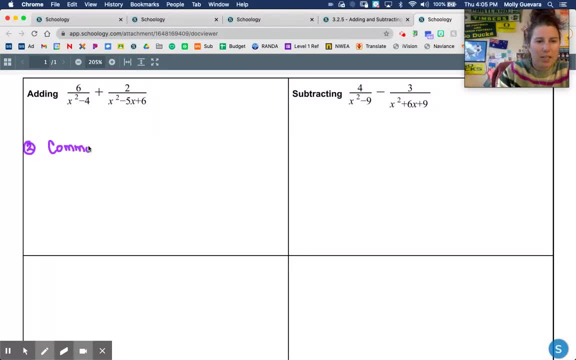 Step two is to find a common denominator. So when we are adding or subtracting from a denominator, we're going to find a common denominator. When we are adding or subtracting from a denominator, we're going to find a common denominator. When we are adding or subtracting from a denominator, we have to have a common denominator. 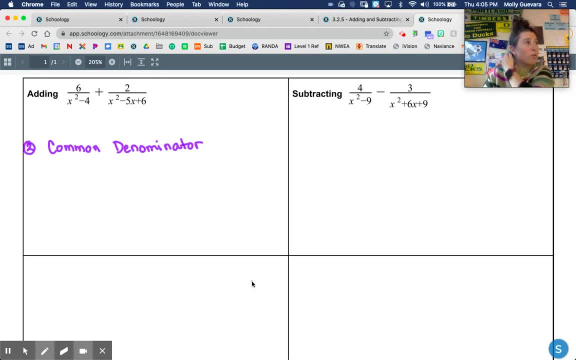 If we don't, we're not able to add them. Okay, so this is the difference between adding, subtracting and multiplying. dividing- Okay, multiplying and dividing. I didn't need a common denominator: Adding, subtracting, I do. 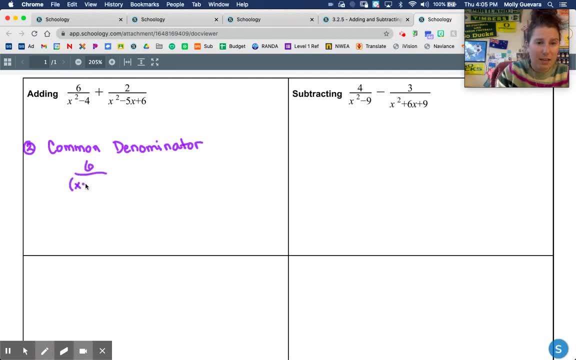 So here the factored form I had here was six, Then I had x minus two, x plus two, And then plus two, And then on the bottom here I have x plus two. I had x minus three, x minus two. 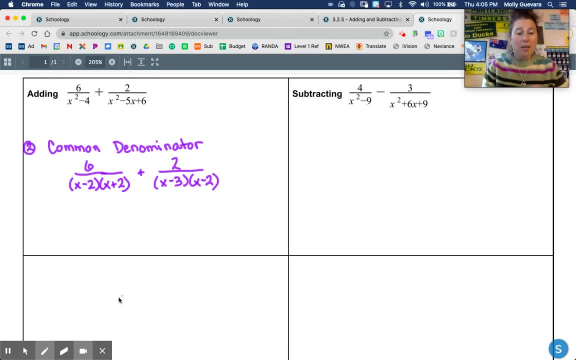 Okay. so when we're finding a common denominator, a couple things have to happen. One, I'm only allowed to add things to my fractions, I'm not allowed to take anything away. So when I look here, I notice that I have an x minus two in both. 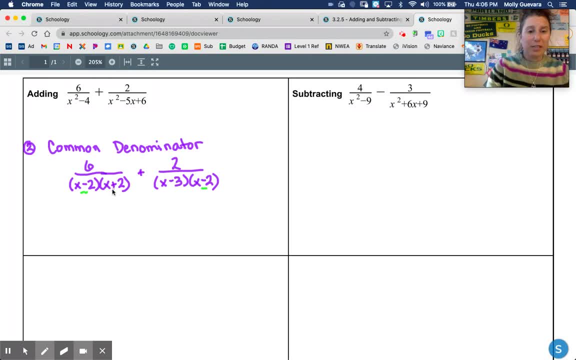 That's good, Okay, that's a good sign. But over here I have an x plus two And over here I don't, So I'm going to subtract, So I'm going to have to add an x plus two onto this side. 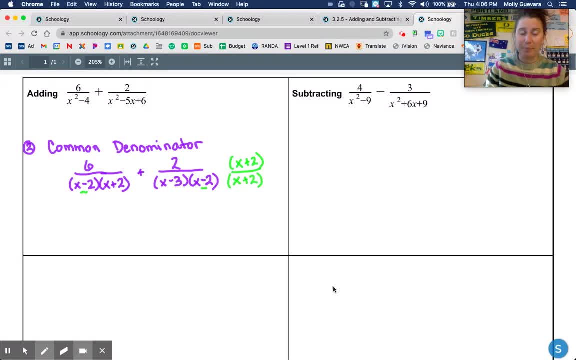 And if I add it to the top, I also have to add it to the bottom, Okay. Or the other way around: If I add it to the bottom, I also have to add it to the top, Okay. So now I have an x plus two in both. 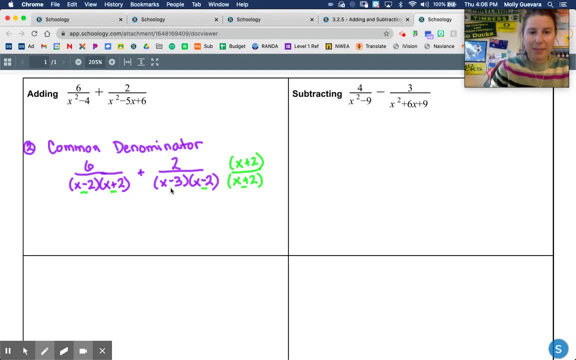 And that's good. Then over here on the right I have an x minus three, but I don't have one over here. So again, I'm going to have to multiply in an x minus three, both to the top And the bottom. 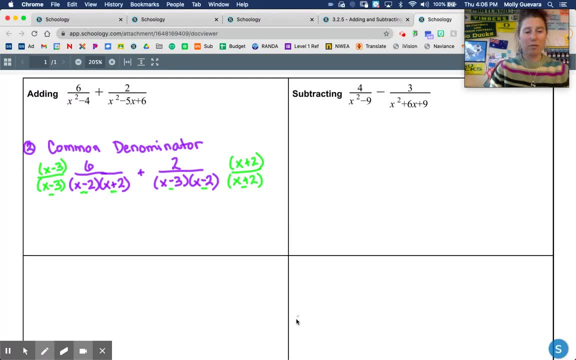 So now I have an x minus three in both. So now I have a common denominator right: X minus three is in both, X minus two is in both, X plus two is in both. So when I go back now, my third step is to simplify that. 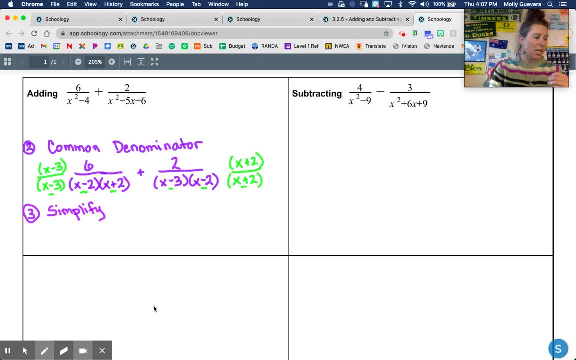 And what that looks like. I am not going to actually distribute out anything on the bottom, So on the bottom I'm just going to leave it as x minus three, x minus two, x plus two. Now, on the top, I can go ahead and distribute. 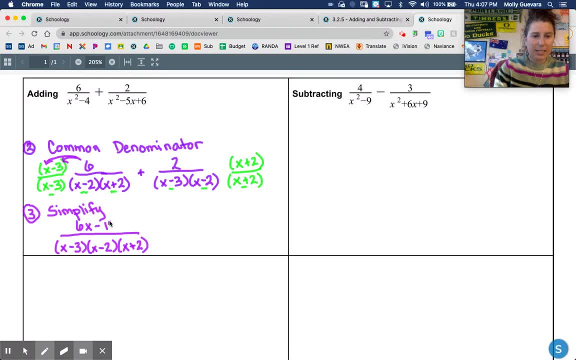 So I get six x minus 18, because I distributed the six to both the x and the negative three. Okay, And then for my second fraction, I'm going to have the same thing. I have an x minus three. I like to write them in the same order as each other. 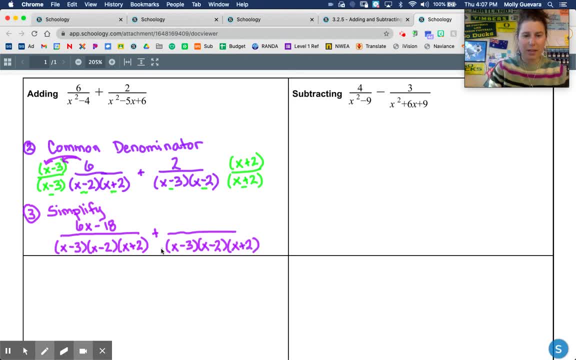 so I can clearly see that there's a common denominator, right. So I have x minus threes, then x minus twos, then x plus twos. So I can clearly see, And then I can distribute this too. So that gives me two x plus four. 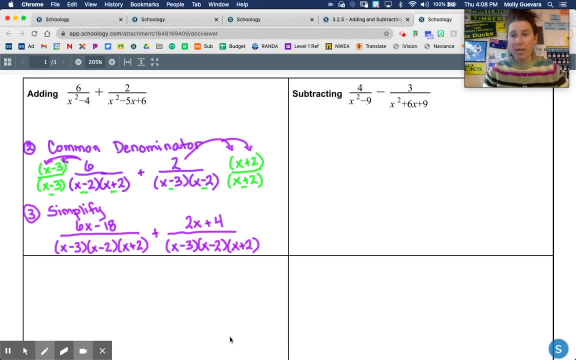 Okay, Okay, So now I have a common denominator. So now I have a common denominator, I can move on to my step four, which is just to add. And when I add fractions, the bottom stays the same. Right, So I have x minus three, x minus two, x plus two. 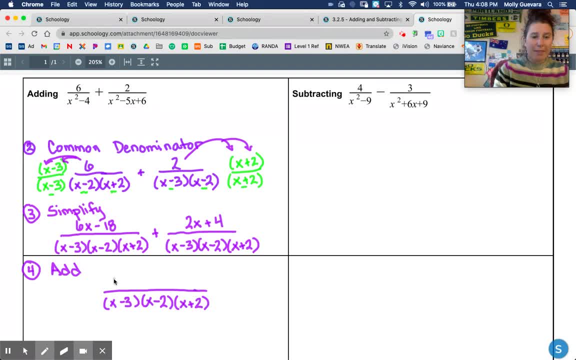 So that just becomes the denominator, And then I'm going to add the top. So six x minus 18 plus two x, X plus four, Which then I can simplify right. So six x plus two x is eight x Negative. 18 plus four is negative 14.. 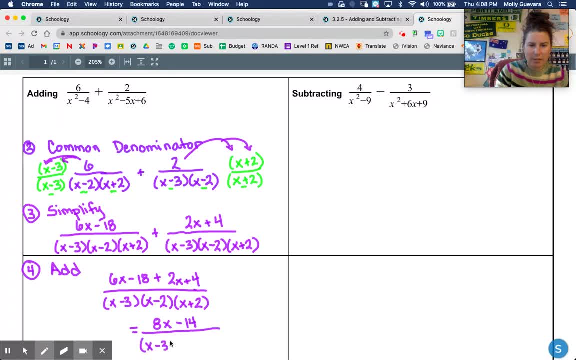 And again, that is still over x minus three, x minus two, x plus two. So I'm going to have to erase this, to scroll down, Or here I'll just write it over to the right. But just know that you want to write it down here, right? 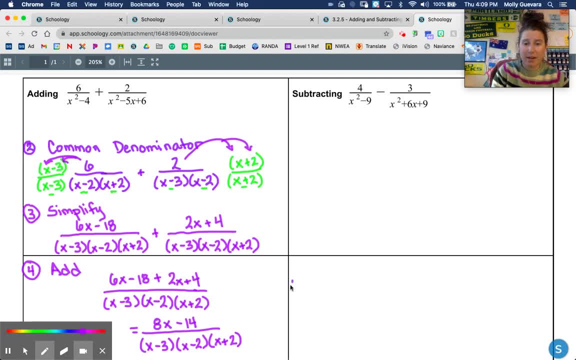 Step five: Okay, But step five says So again on your paper. instead of writing it over here on the right, you just want to write it underneath this. So step five says: factor again If possible. If it's not possible, that's okay. 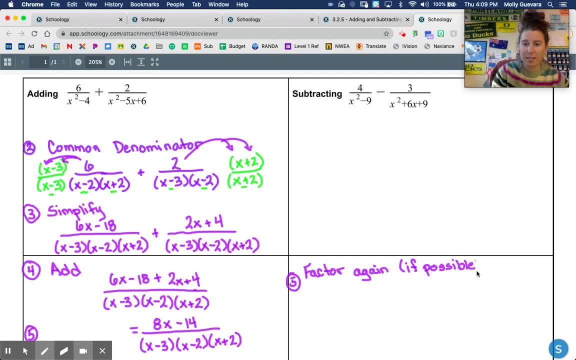 Sometimes it is, Sometimes it isn't, And see if anything cancels, Anything cancels. So in this case I can factor the top right I am. Two goes into both of those, I can take out a two And I'm left with four x minus seven. 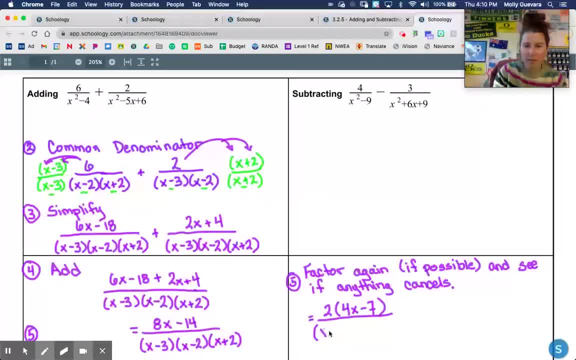 On the top And then on the bottom, I still have x minus three, x minus two, x plus two. So what I was looking for was maybe this four x minus seven could cancel with one of these, But in this case it can't. 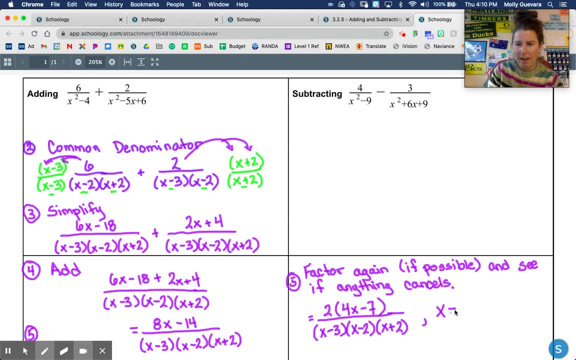 So that's fine. So that's my final answer. And then we just can't forget to always include what values x is not allowed to equal. So here I cannot have three, Because if I plug in three I'll get three. 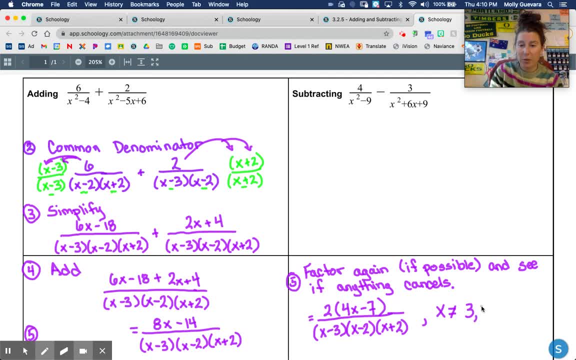 So I can't have three, So I can't get zero. I also cannot have two, Because if I plug in two here, I will get zero. And I cannot have negative two, Because if I plug in negative two, I will get zero. 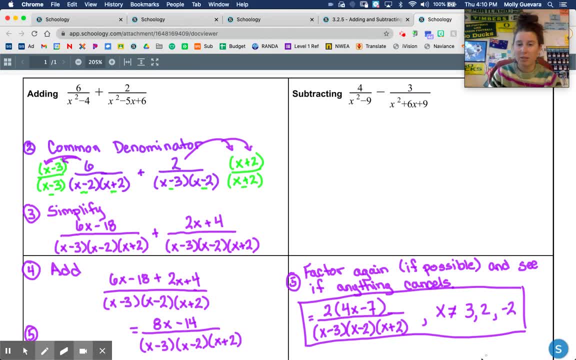 Okay, And there is my answer. So kind of similar to multiplying, dividing, Except you have to get that common denominator. And that's really kind of the tricky part here Is getting that common denominator. Let's look at example two, Which is all about subtracting. 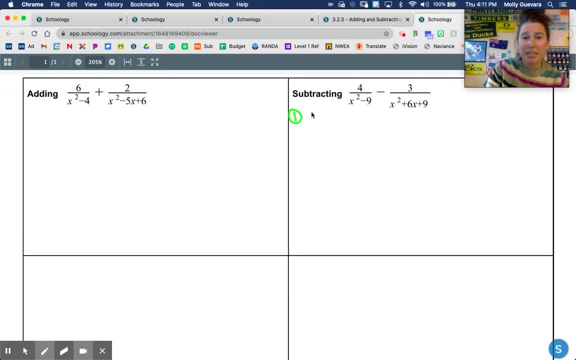 Ooh, that's a bright color. Okay, First step, same thing: Factor everything. Factor anything and everything that you can. So in this case, four doesn't factor X squared minus nine factors to x plus three, X minus three. 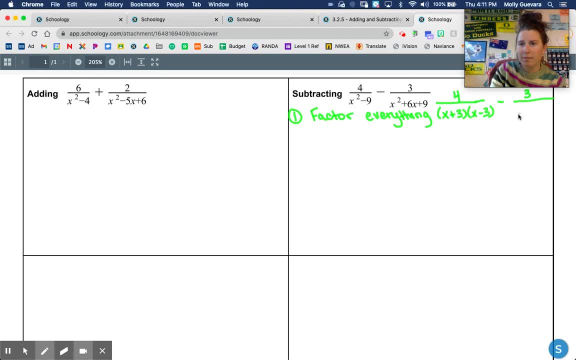 Minus three doesn't factor, And x squared plus six, x plus nine, factors to x plus three And x plus three. So there's step one Factored everything. Step two is that I need to get a common denominator. So again, similar to what I said with multiplying, dividing. 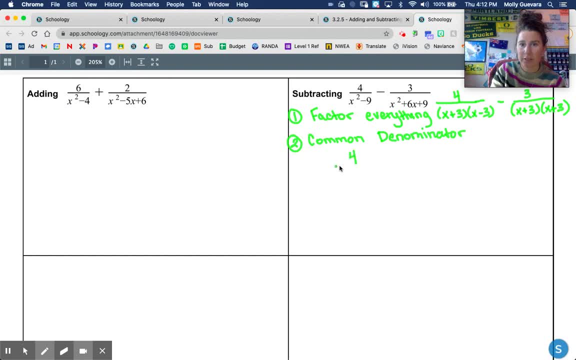 You don't always have to write like this over and over and, over and over, But we are in this case because for notes, it's helpful to see each step very clearly written out. Okay, But like normally, I would probably combine step one and two here. 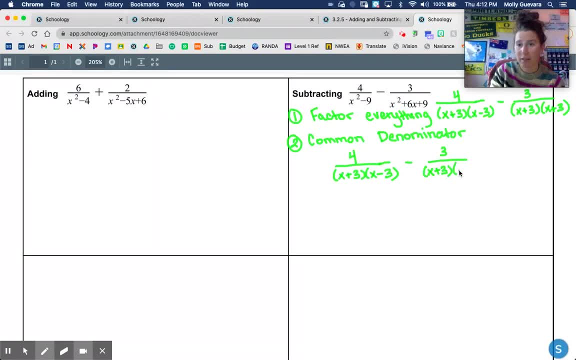 So I didn't have to write it twice. Okay, So here is my factored form, And I'm looking for a common denominator. So I see an x plus three in both. That's good, Right. Here I see an x minus three. 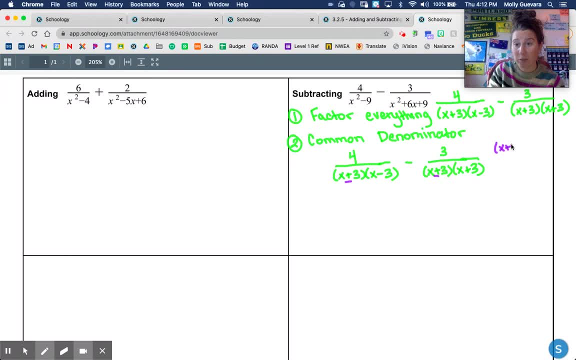 And here I don't, So I'm going to have to multiply in an x minus three. Or, wow, I said x minus three and I wrote x plus three. I'm so sorry, We're going to have to add in an x minus three. 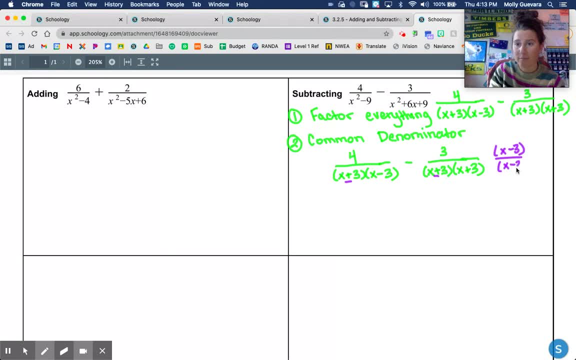 To both the top and the bottom Right, So now that's common in both. And then on the right here I have another x plus three that I don't have over here, So I am also going to have to multiply in another x plus three. 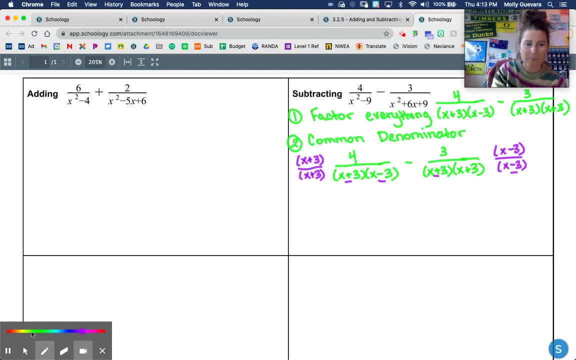 I'm supposed to have two of those and I only have one. Okay, So what that does is that allows me to figure out what that common denominator is. Okay, So now I can go ahead and simplify. So on the bottom, I'm going to have those x plus threes. 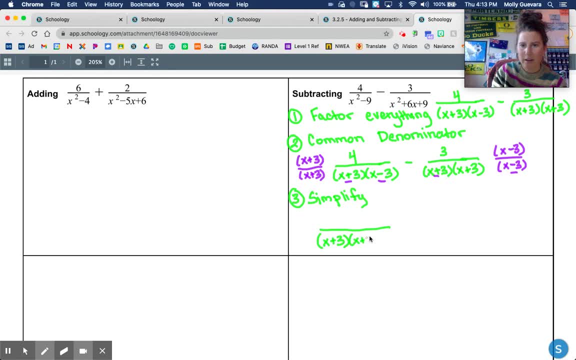 And I have two of them. So x plus three, x plus three, x minus three. And then on the top, don't forget, I can distribute. So four times x is four x, Four times three is twelve. Okay, So now I can go ahead and simplify. 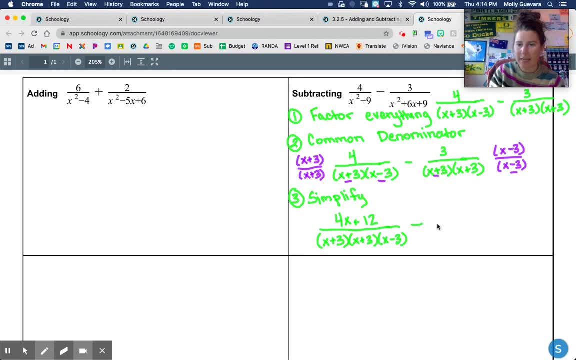 So now I can go ahead and simplify. Okay, then this is minus, and again I like to do the bottom first. just because I already know what's supposed to be there, I don't have to like think about anything. I've already found my common denominator. so there's the bottom, and 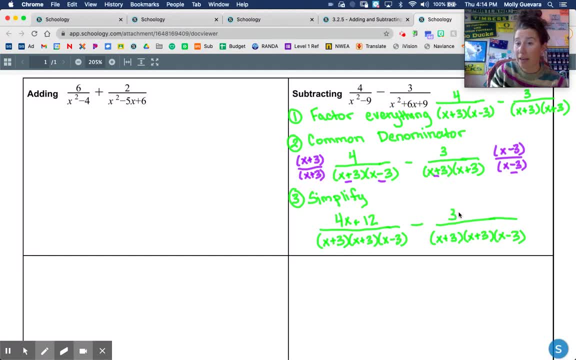 then the top I can distribute. so I have 3x minus 9. okay, step 4 here- and this is where it's a little bit different- is that I need to subtract, and I'm gonna make a very big point of this. we have to distribute, distribute the negative. 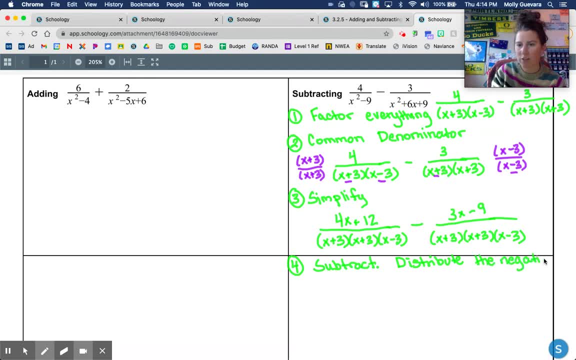 because we are subtracting, we have to distribute the negative. because we are subtracting, we have to distribute the negative. because we are subtracting, we distribute the negative right. we distribute the negative. that's subtracting. we distribute the negative. that's subtracting. we distribute the negative. that's right here in the middle, the, the. 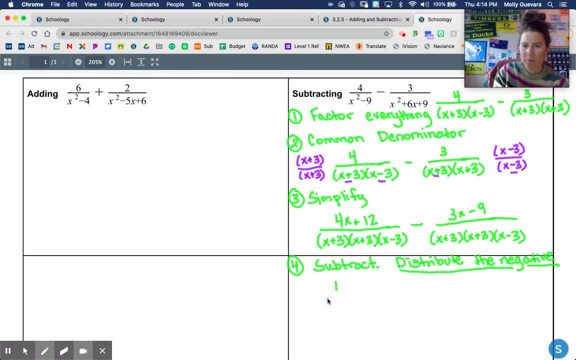 right here in the middle the. the right here in the middle the the minus sign. so this becomes actually let's minus sign. so this becomes actually let's minus sign. so this becomes actually: let's write the bottom and X plus 3 X. write the bottom and X plus 3 X. 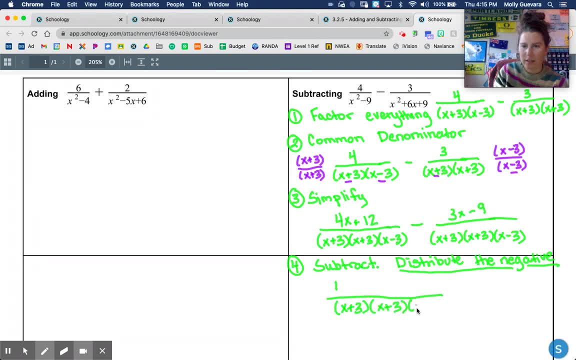 write the bottom and X plus 3, X plus 3, X minus 3, so I have 4x plus 12 plus 3 x minus 3, so I have 4x plus 12 plus 3 x minus 3, so I have 4x plus 12. now, when I'm minus, I have to put that: 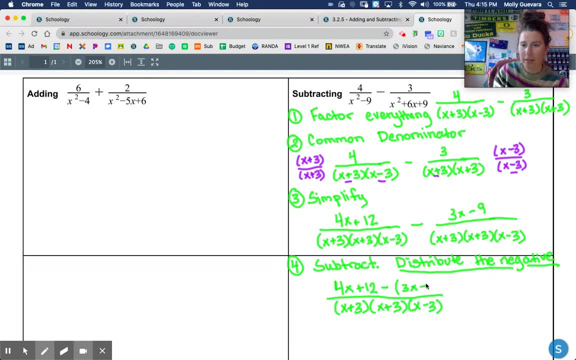 now when I'm minus, I have to put that. now when I'm minus, I have to put that second term in parentheses: 3x minus 9: I. second term in parentheses: 3x minus 9: I. second term in parentheses: 3x minus 9. I have to put it in parentheses because 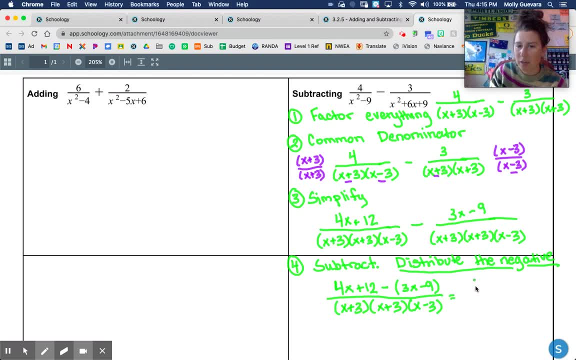 have to put it in parentheses, because have to put it in parentheses because I'm gonna end up distributing, right, so I'm gonna end up distributing right, so I'm gonna end up distributing right, so it becomes 4x plus 12 minus 3x plus 9. 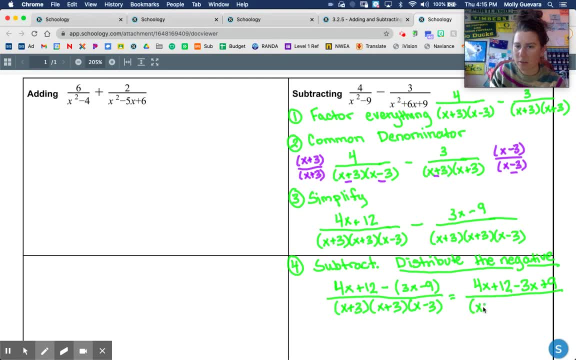 it becomes 4x plus 12 minus 3x plus 9. it becomes 4x plus 12 minus 3x plus 9. you see that, so I distributed those the. you see that. so I distributed those the. you see that, so I distributed those. the minus sign and then the bottom still. 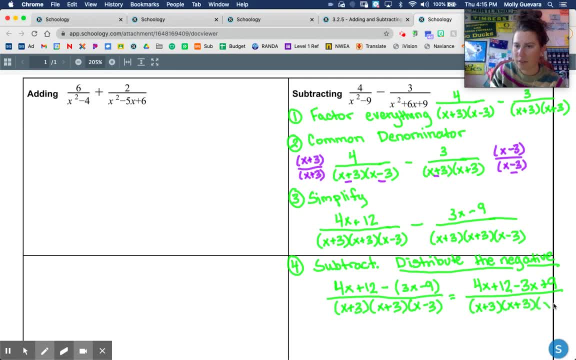 minus sign, and then the bottom still minus sign, and then the bottom still the same. so you just have to be very the same. so you just have to be very the same. so you just have to be very careful about whatever your second, careful about whatever your second. 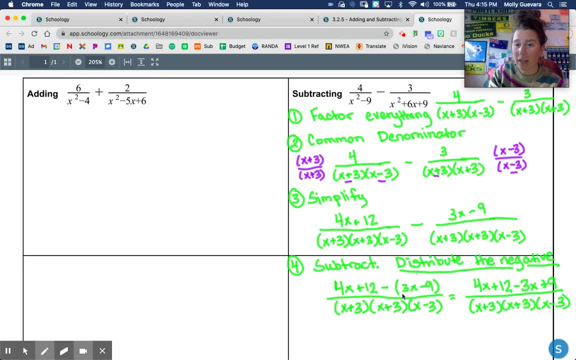 careful about whatever. your second fraction is that you are distributing. fraction is that you are distributing. fraction is that you are distributing this negative in. okay, so I distributed this negative in. okay, so I distributed this negative in. okay, so I distributed this negative. so, if I simplify this, 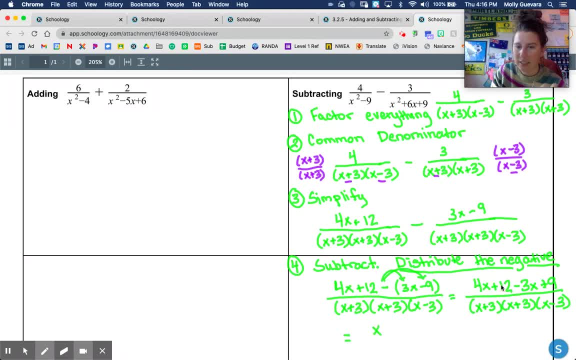 this negative. so if I simplify this, this negative, so if I simplify this again, 4x minus 3x is just X, 12 plus 9. again, 4x minus 3x is just X, 12 plus 9. again, 4x minus 3x is just X, 12 plus 9 is 21, so I have X plus 21 over this. 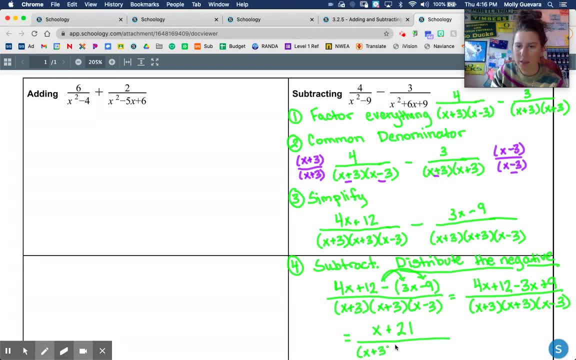 is 21, so I have X plus 21 over this is 21, so I have X plus 21 over this whole thing, whole thing, whole thing, which is X plus 3x plus 3x minus 3, and then the last step, step 5: which is X plus 3x plus 3x minus 3, and then the last step, step 5, which is X plus 3x plus 3x minus 3, and then the last step, step 5, again, you would write it over here: 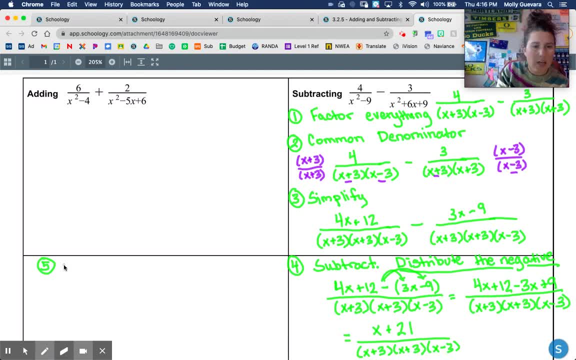 again. you would write it over here again. you would write it over here underneath step 4, but I just don't have underneath step 4, but I just don't have underneath step 4, but I just don't have room. um, so in this case, right, I cannot. 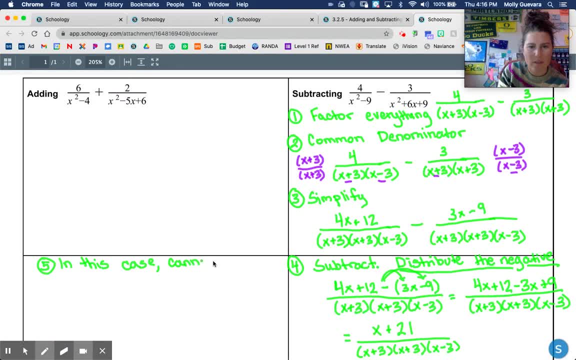 room um. so in this case, right, I cannot room um. so in this case, right, I cannot factor. factor again: X plus 21 does not factor. so that just X plus 21 does not factor. so that just X plus 21 does not factor. so that just means that that's my final answer. so X. 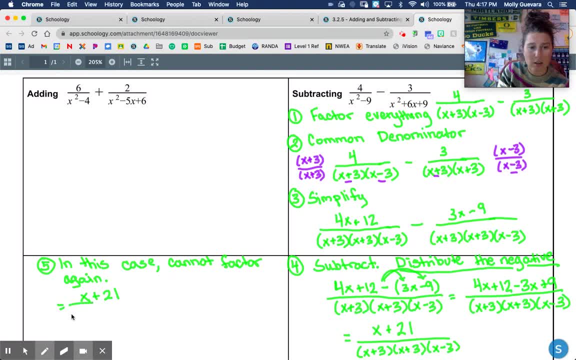 means that that's my final answer. so X means that that's my final answer. so X plus 21 all over now and you can write plus 21 all over now and you can write plus 21 all over now and you can write it X plus 3x plus 3x minus 3, or you can. 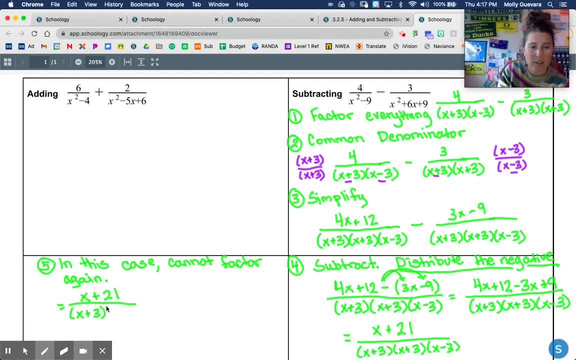 it X plus 3x plus 3x minus 3, or you can it X plus 3x plus 3x minus 3, or you can write it X plus 3 squared, since we have. write it X plus 3 squared, since we have. 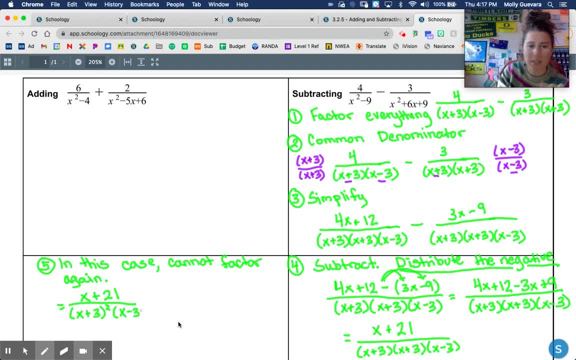 write it X plus 3 squared. since we have two of them: X minus 3. that's another two of them X minus 3. that's another two of them X minus 3. that's another option as well. either one of these two option as well, either one of these two. 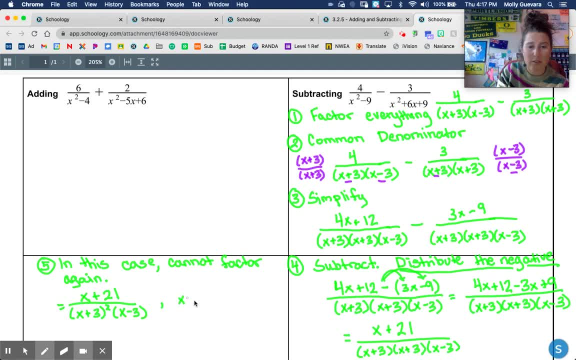 option as well. either one of these two would be okay, and then don't forget to would be okay, and then don't forget to would be okay. and then don't forget to include the values that X is not allowed. include the values that X is not allowed. 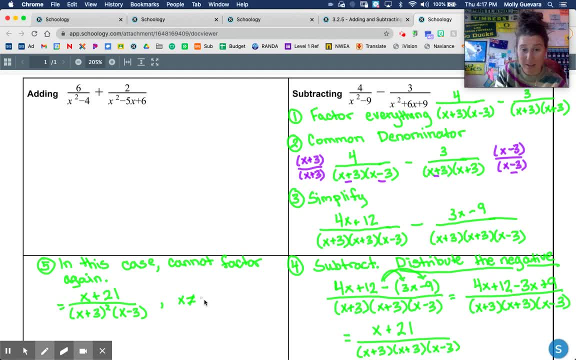 include the values that X is not allowed to equal. so here X cannot be negative to equal. so here X cannot be negative to equal. so here X cannot be negative. 3, because that would give you 0 and X. 3, because that would give you 0 and X. 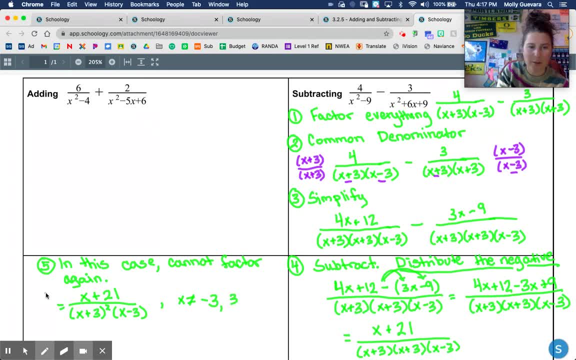 3 because that would give you 0 and X cannot be positive. 3 because that would cannot be positive. 3 because that would cannot be positive. 3 because that would get you 0. and there is my answer. so: 0 and there is my answer. so. 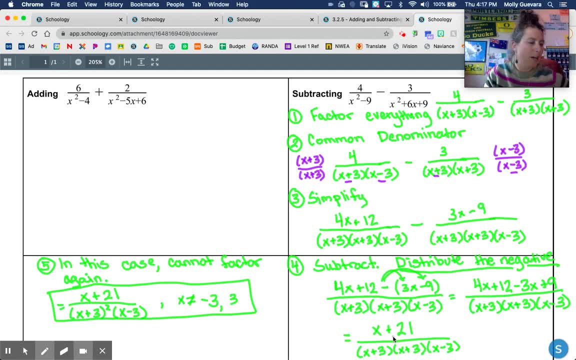 0 and there is my answer. so twice it's just your choice. um, okay, so I twice. it's just your choice. um, okay, so I twice. it's just your choice. um, okay, so I know that was kind of fast if you have. know that was kind of fast if you have. 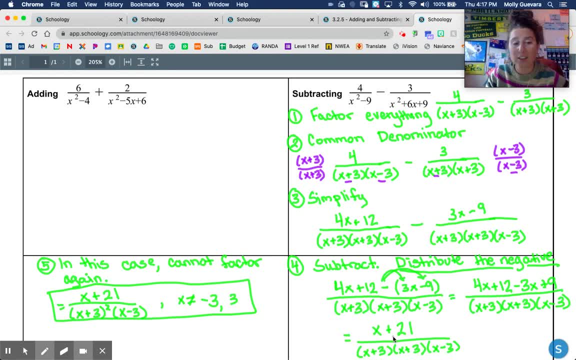 know, that was kind of fast. if you have any questions, or you get stuck on this, any questions, or you get stuck on this, any questions, or you get stuck on this. or you need anything at all, just make. or you need anything at all, just make. or you need anything at all, just make sure that you reach out to me. let me. 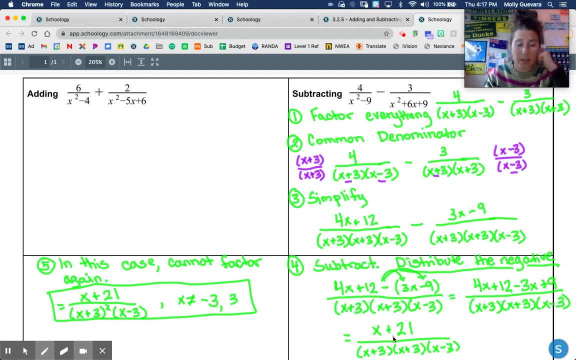 sure that you reach out to me. let me sure that you reach out to me. let me know we can go over whatever we need to know. we can go over whatever we need to know. we can go over whatever we need to go over. I can help you in any way, but